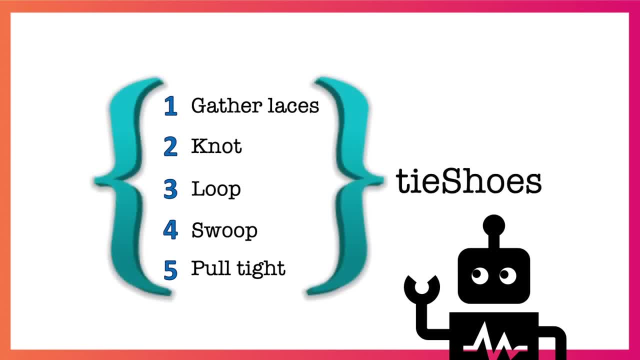 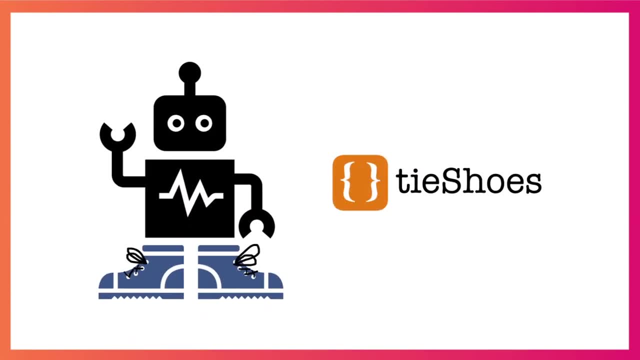 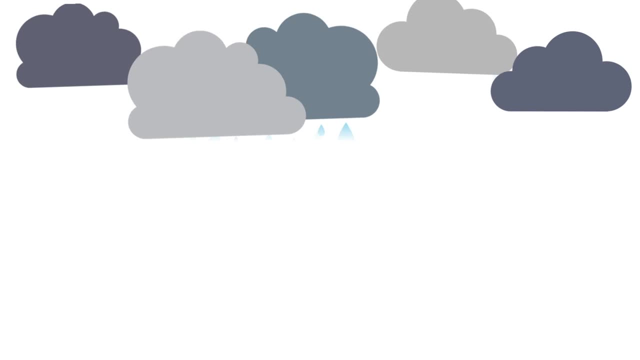 commands, Then give the action a name so it's easy to tell the computer to repeat it later. Now you can simply use the function name tie shoes anytime and your computer will complete the exact same action. So why are functions so important? Well, the main reason is that they help keep your code dry. Dry means don't repeat. 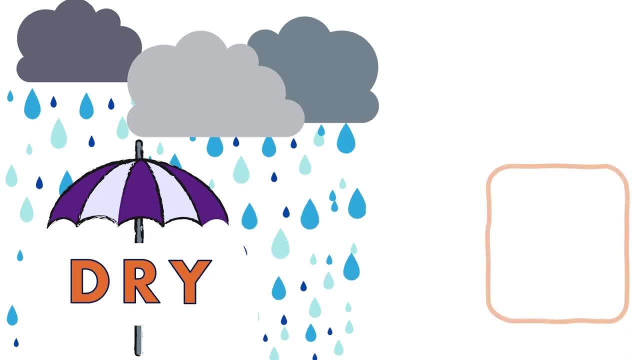 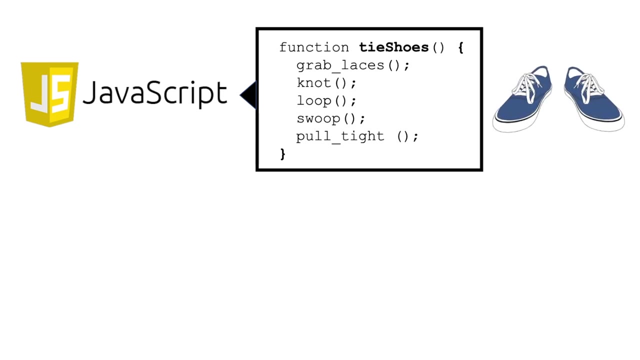 yourself. Cutting out repeating commands helps to minimize bugs, keeps code short and saves programming time. You might be wondering: what does a function look like in code? In JavaScript, a function looks like this. Here's an example of our tie shoes function we used earlier: The sequence of steps you want the computer to. 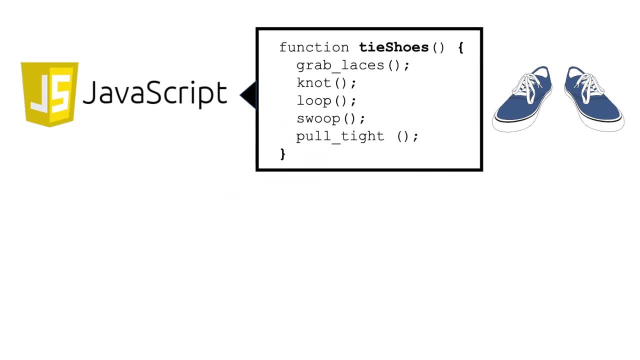 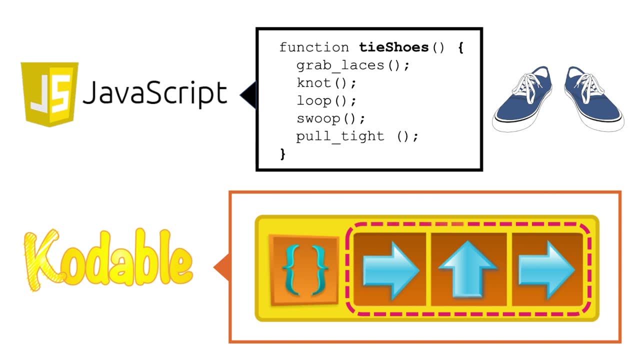 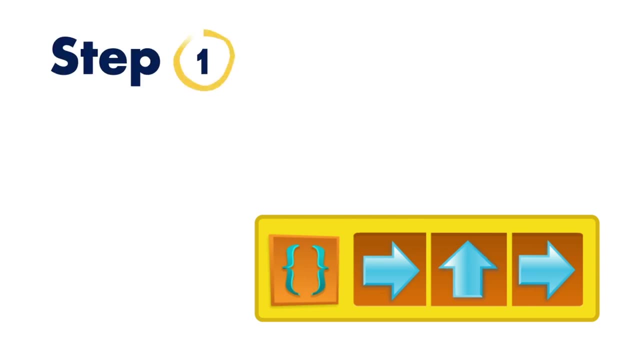 repeat is stored between these two In code. this is what a function looks like. The sequence of steps you want your fuzz to repeat are stored in the function's bin with the same squiggly symbol. There are two main steps to create a function. Step one: define it In code. this means choosing: 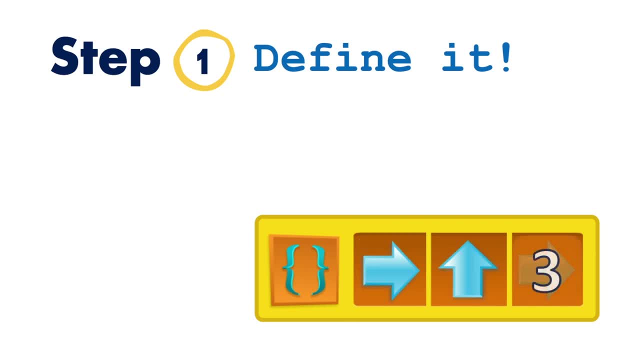 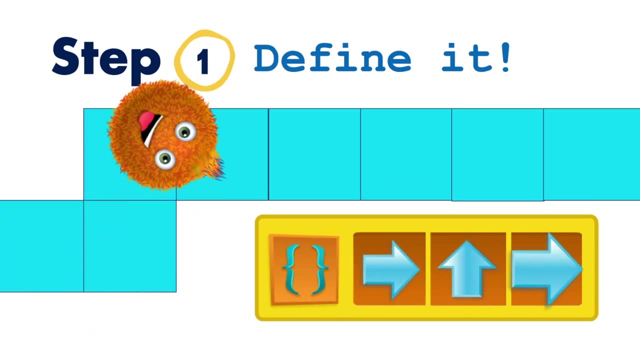 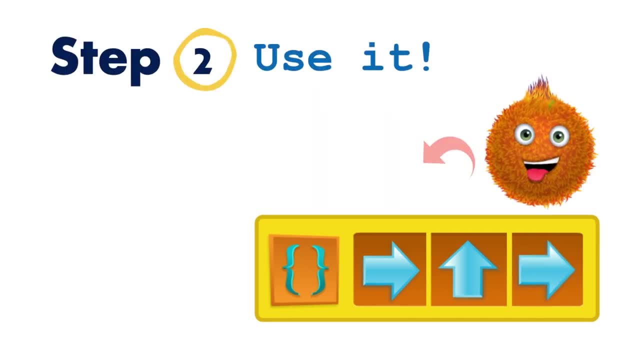 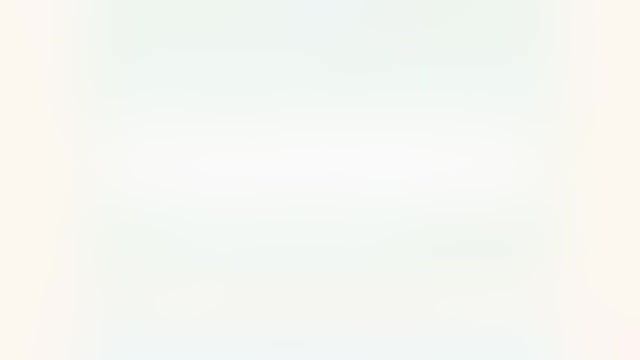 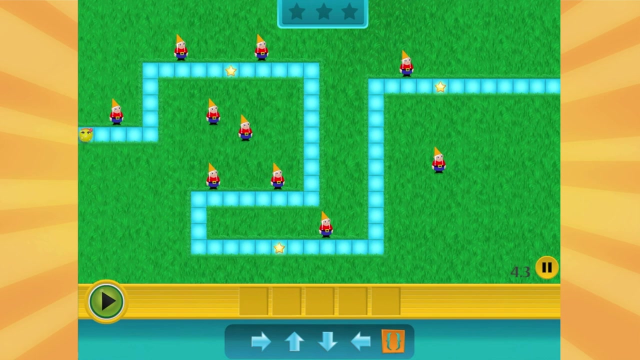 function instead of dragging out those same commands again. Now it's your turn. Use the function command in Codable to store a series of steps that repeat throughout a level. Start by looking for patterns Here. I want my fuzz to move right up, right. I notice later in the maze the fuzz will repeat these again. I will. 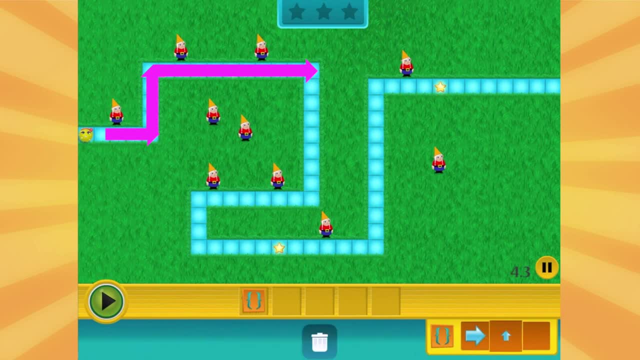 put these three commands in a function. right up right, Let's work through the rest of the level. Now I don't have space in my program to drag out the same arrow commands again. That's okay. I just need the function block to move my fuzz right up right, Let's.